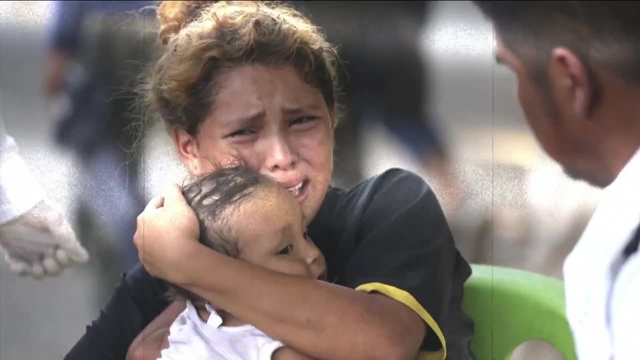 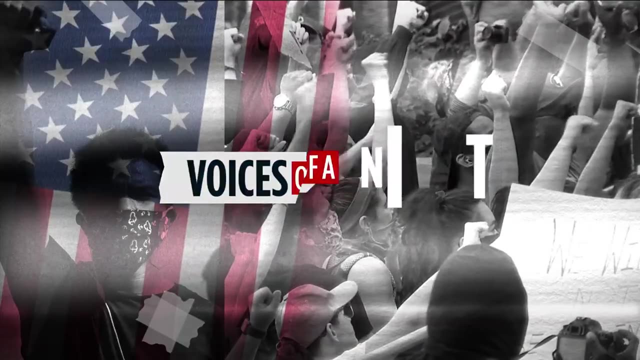 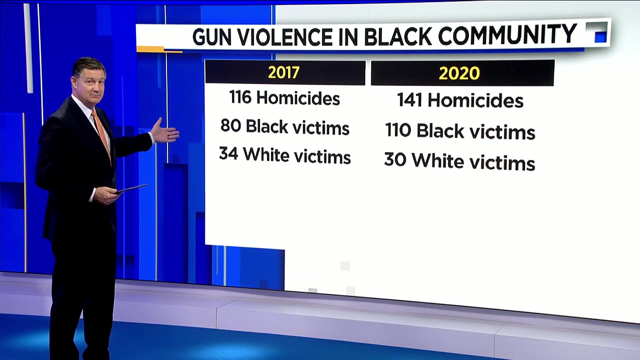 Voices of a Nation. records show gun violence in Jacksonville continues to disproportionately impact the black community at an alarming rate. According to the Jacksonville Sheriff's Office, in 2017 there were 116 homicides, 80 black victims versus 34 white victims In 2020. there. 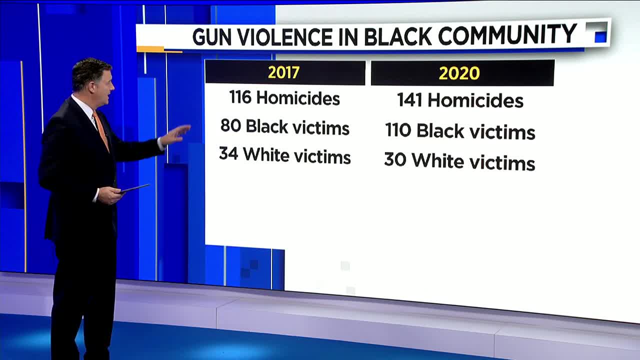 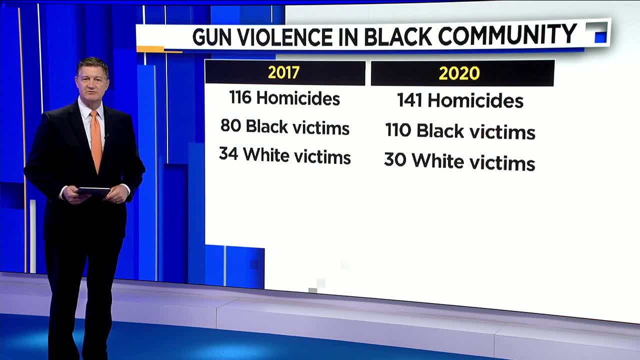 were 147, 41 homicides, that is, 110 of the victims were black, 30 were white. News for Jaxx reporter Zach Lashway is speaking with two families affected by gun violence and tonight they're showing us what they're doing to try to ensure other parents won't have to deal with the. 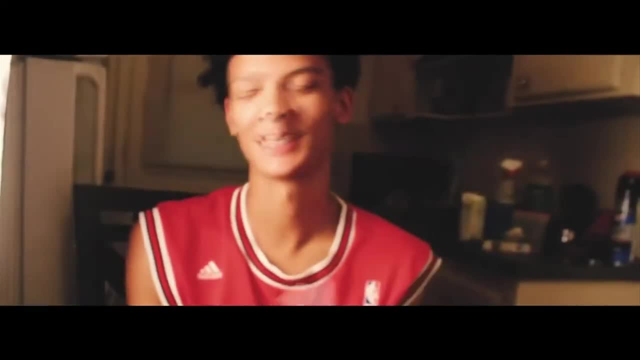 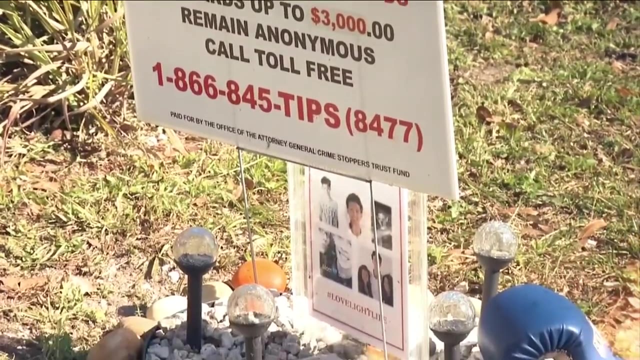 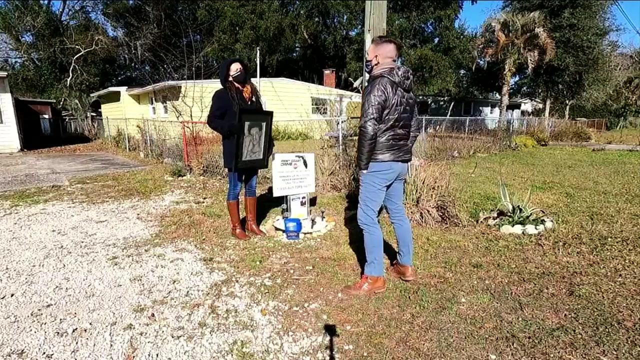 pain of losing a child. Four years ago and one week to the day, Maurice had just turned 18. two days before he was shot, The Hobbs family went from celebrating to mourning. January 26, 2017 was the day that he began to live through me. A fence, now red, marks the spot where 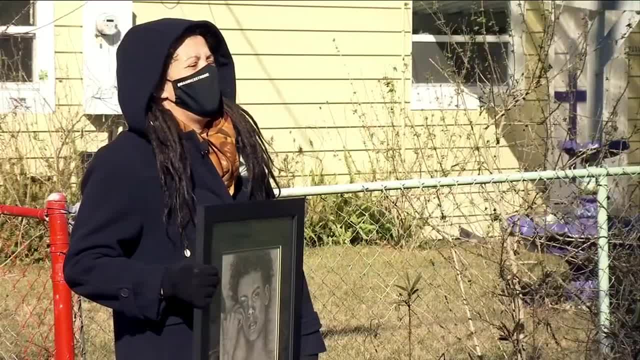 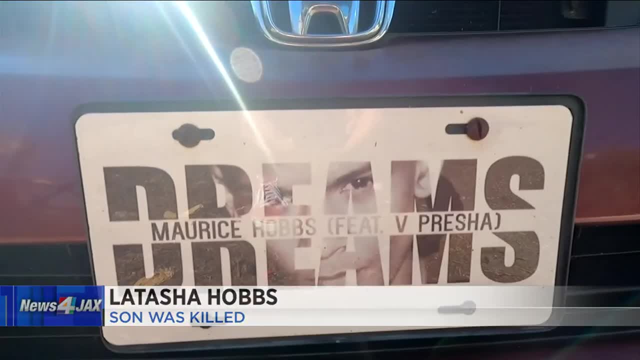 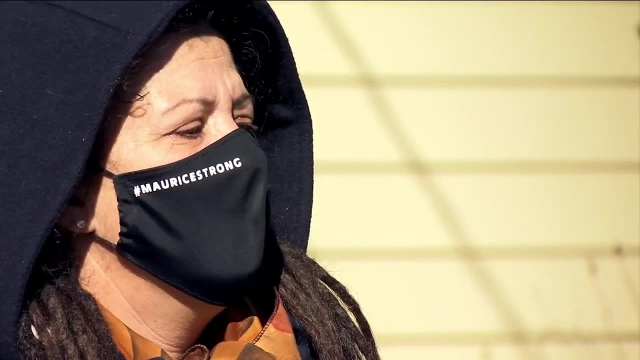 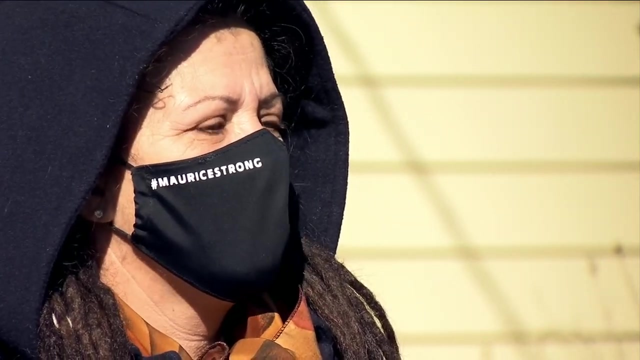 18-year-old Maurice Hobbs took his last breath. I made a wrong turn and moments later shots ring. Hobbs was driving to pick up Maurice. Maybe, had I just went straight and not turned right, he would still be here. It's a struggle. I'm his mother. I live and breathe for my children. 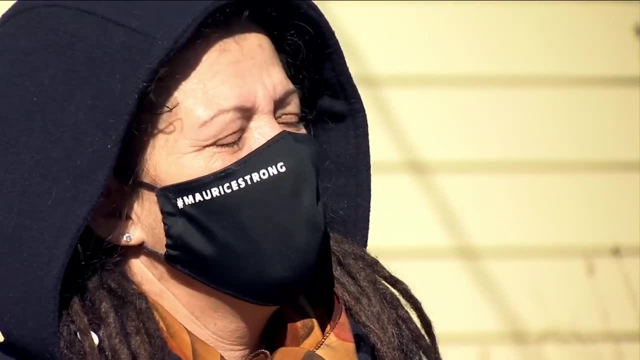 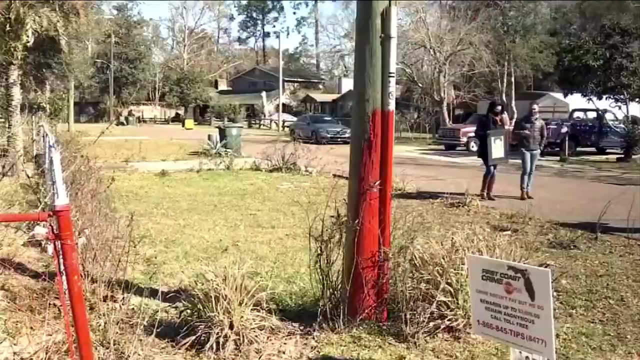 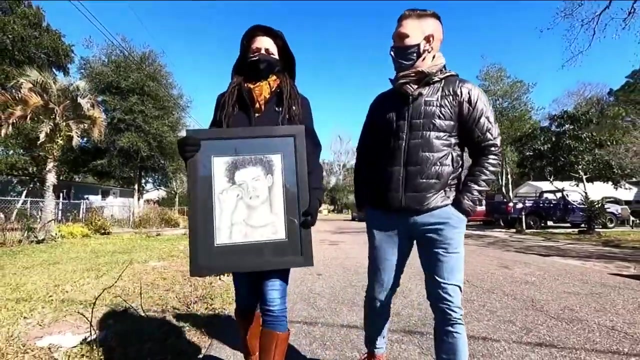 It's my duty, it's my job to protect my children. I feel like I failed him. The mother heard the gunshots that killed her son. This was the street you were not able to find that January night. Yes, it is. You know those responsible for the harm of my son. they may. 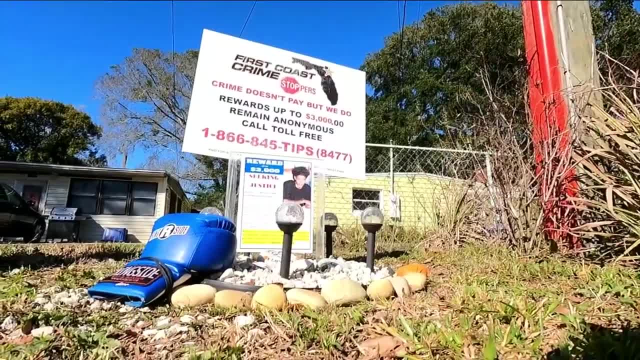